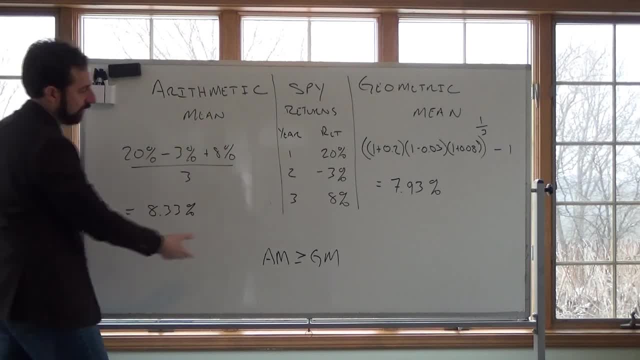 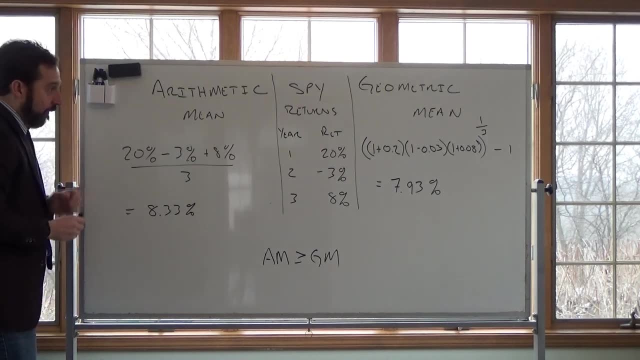 Of course, the easier way of writing that is just simply to sum them up and divide by 3.. So sum up all the returns, divide by the number of years. That gives us 8.33%. Now, when do we use this return? 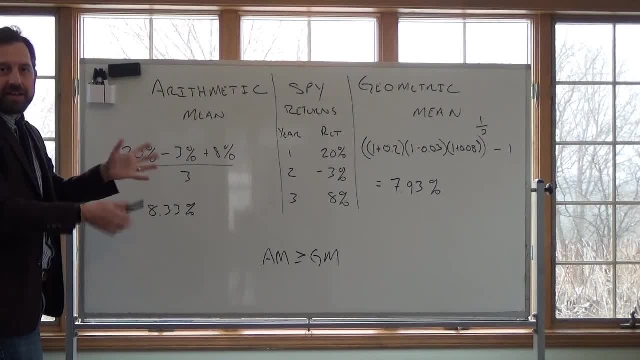 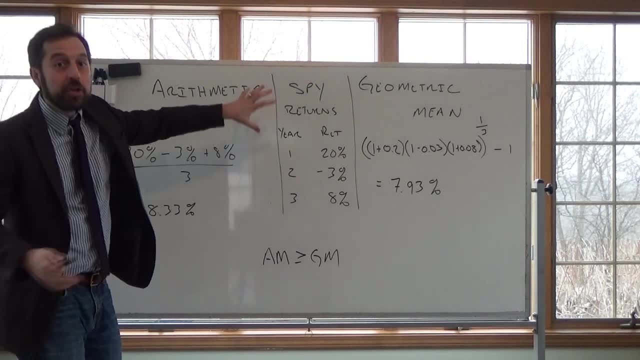 So the big thing here is: I highly recommend Excel will calculate this for you. The calculation of this isn't the problem. The big thing that you want to get from this is: when do you use each type of return? So when is this type of return appropriate? 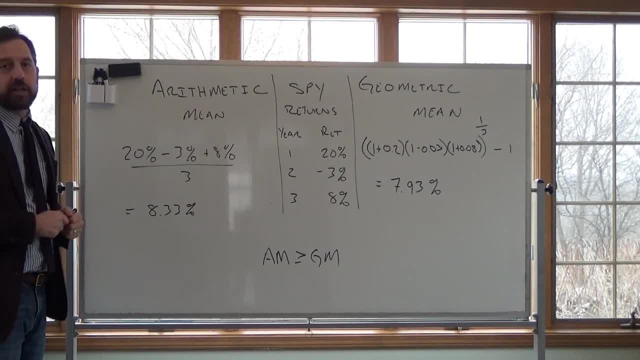 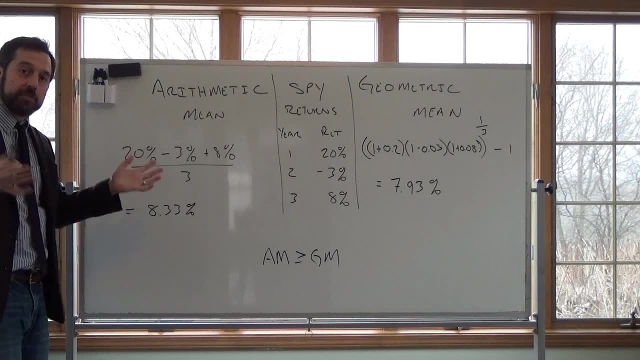 So the idea is, if somebody asked me, what do you expect the market to do next year, Then I would use the arithmetic return. I'd say, okay, I expect. I expect the market to return 8.33%, if I'm going to use a mean for that. 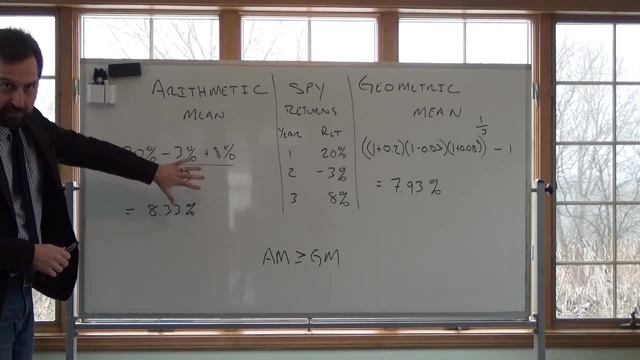 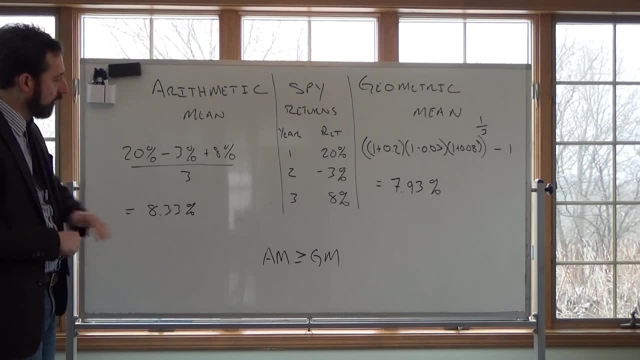 But that would be an appropriate use of an arithmetic mean. So again, the way you would use the arithmetic mean is if somebody said, well, what do you expect the market to do next year, Then we can go with this. Now, the geometric mean answers a different question. 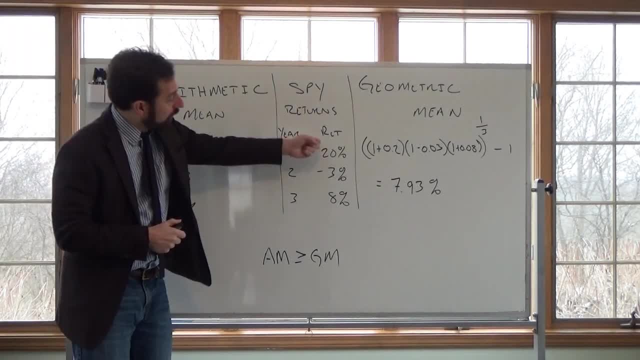 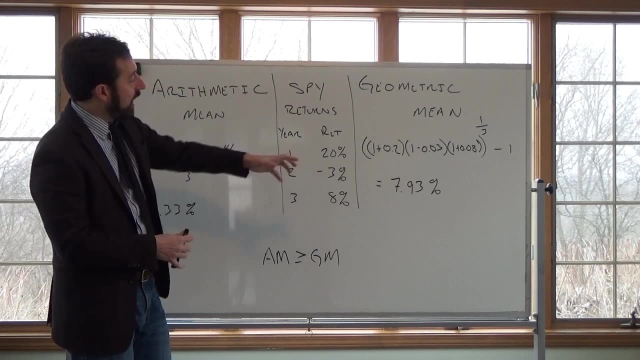 So what the geometric mean is going to answer is: if I own the market over this period, what was my annual return? That is not what the arithmetic mean says. So if we want to get that, Then remember if we invest in the market at the beginning of the first year. 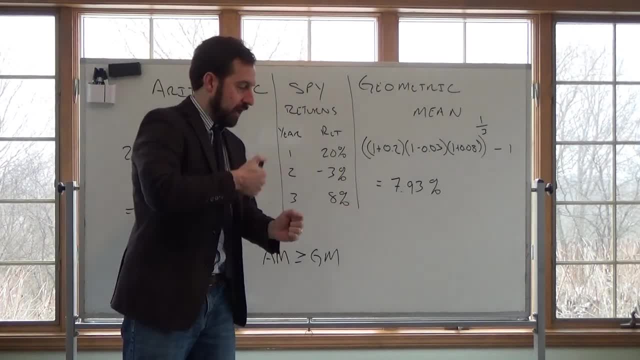 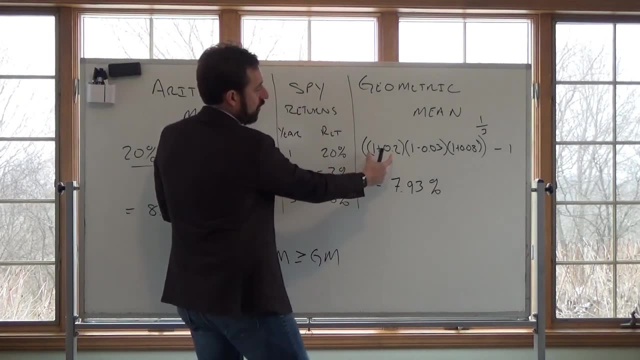 well, our returns are going to compound, right. So what we're going to do with the geometric mean is take into account this compounding. So the idea here is we earn 20% the first year, lose 3% and then we earn 8%. 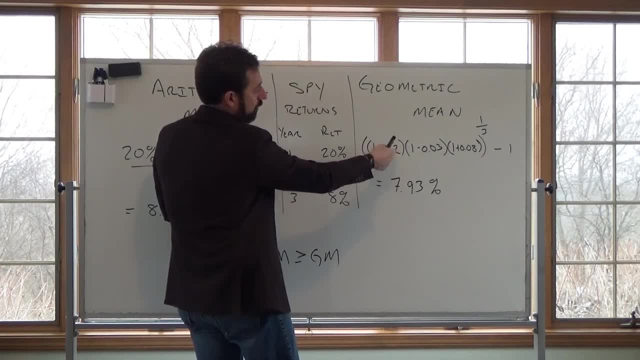 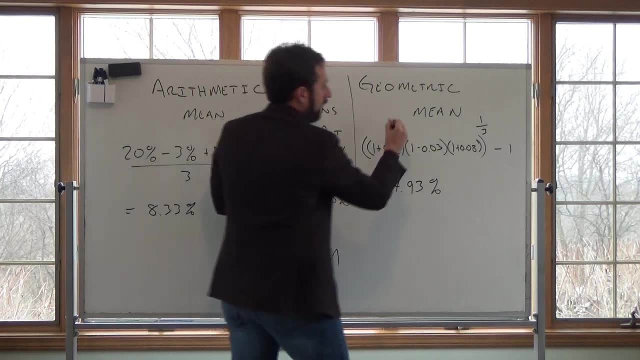 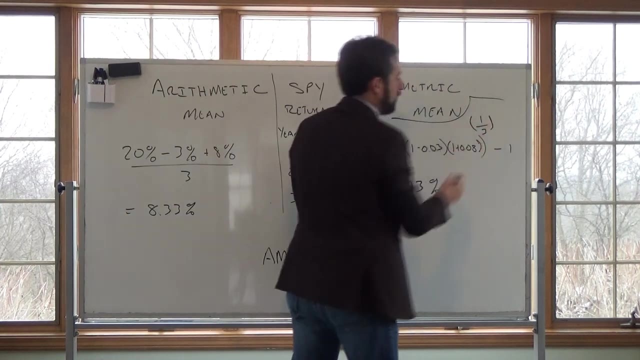 So you know, take into account compounding, we have 1.02 times 0.97 times 1.08.. And then we take the third, the cube root of it, right. So in your calculator this: Well, if I were to enter this in Excel, I would take these three numbers and raise it to the power of one-third. 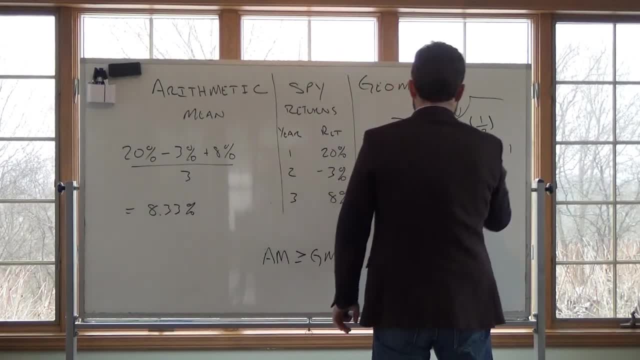 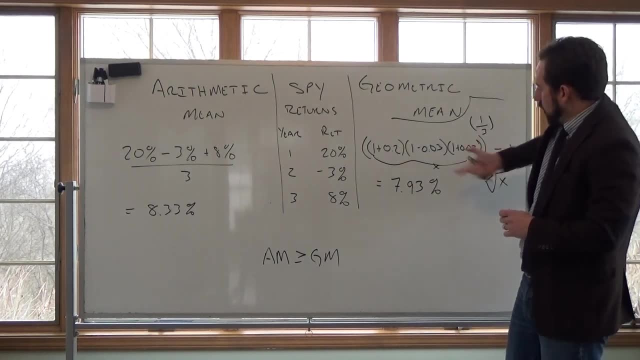 Of course this is. you know, if this number here is x, then this is just the cube root of x. It's another way to write the same thing. So if I take the cube root of this, I get an annual return of 7.93%.